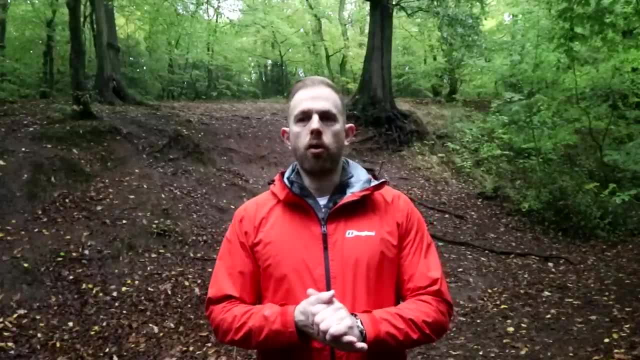 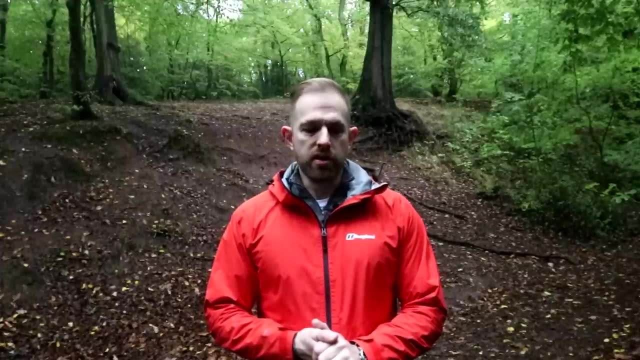 give it a like, Tell me whether it's actually a valuable video or not and if not, I will include some links to some other videos going through global atmospheric circulation. Now, if you're new to the series Sunday morning coffee- our weekly AQA GCSE geography videos- I'm going to 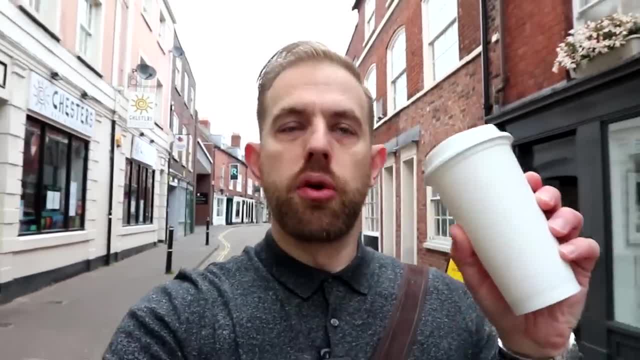 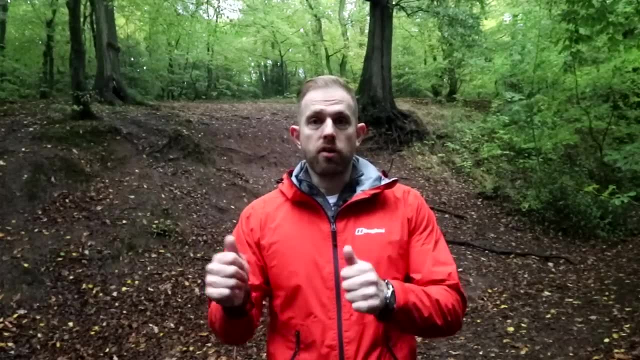 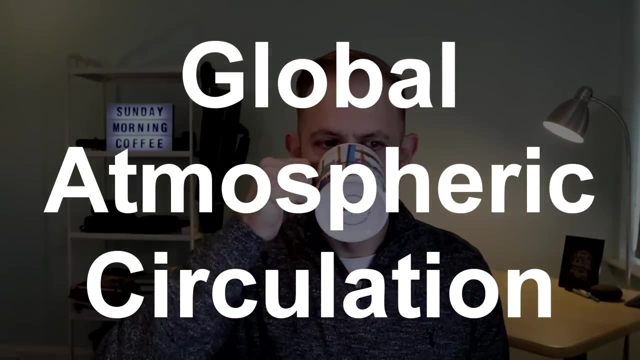 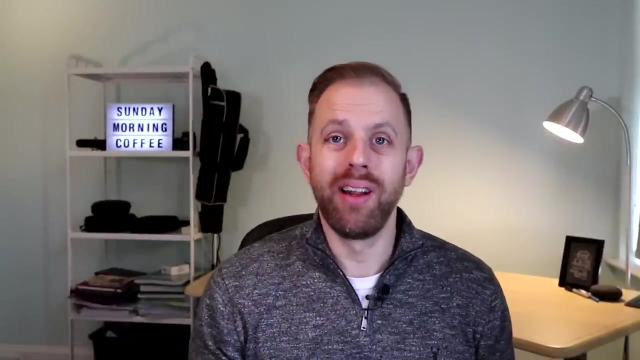 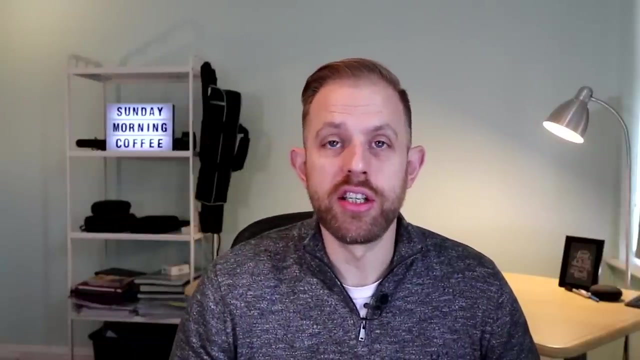 try and go through the entire course. So click the link above in the description: go check out some of the videos. So let's get into global atmospheric circulation. It's a very difficult topic. It's absolutely fine if, as a GCSE student, you find it quite difficult, but just bear with it, Try and 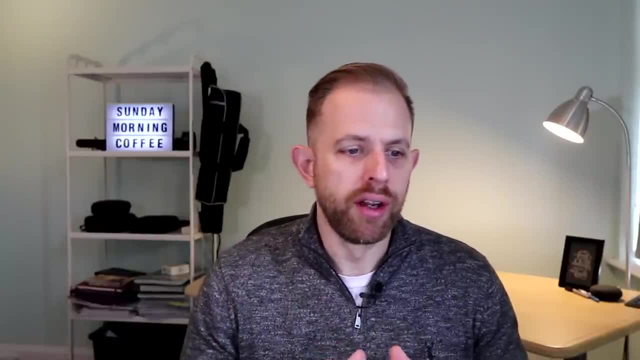 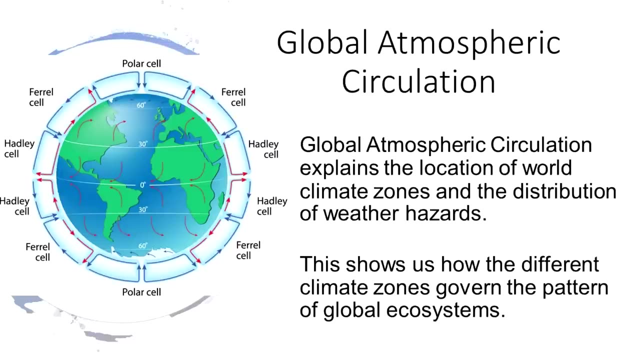 break it down into the different sections. I'm sure you're going to do well with it. Okay, so here's our first definition about what global atmospheric circulation actually is. Global atmospheric circulation explains the location of world climate zones and the distribution of weather hazards. This shows us how the different climate zones govern the pattern of 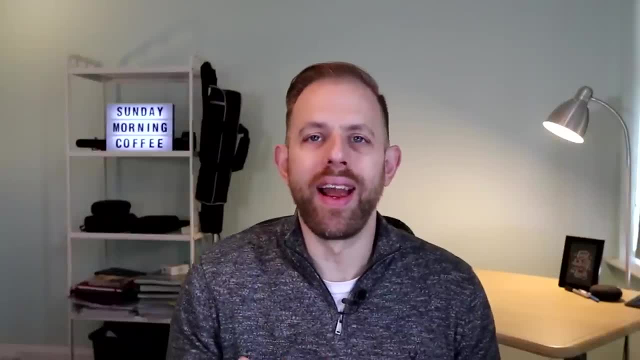 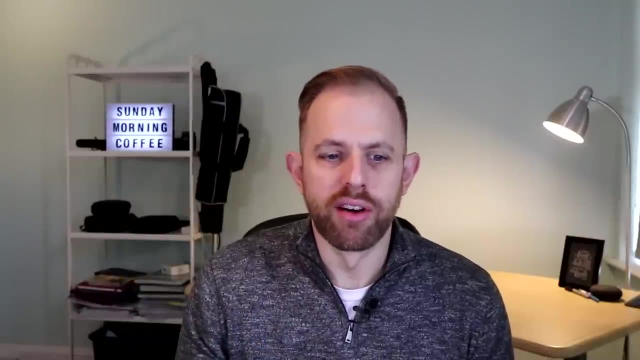 global ecosystems. So basically, this is a way of trying to explain why we get different climates around the world and why we get those different weather patterns and weather hazards around the world, as well as the different ecosystems. So here's our first definition about what global 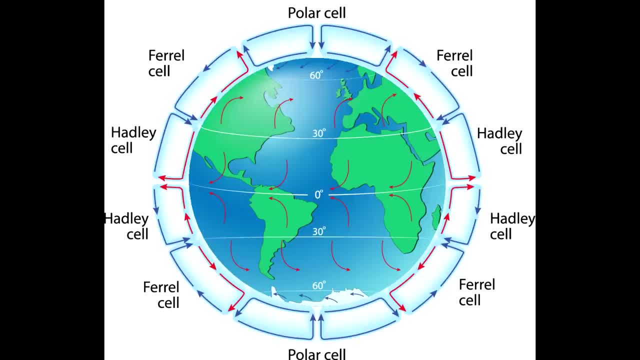 atmospheric circulation is. So this is our model, our diagram of global atmospheric circulation, and it looks very complicated, but as soon as we start breaking it down into different sections, it's going to make more sense. So the major thing we want to look at first is the different latitudes around the 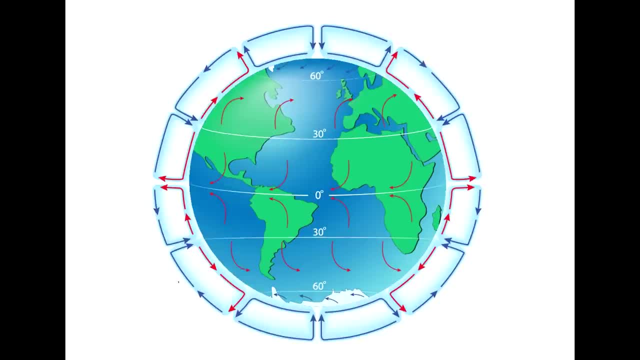 earth, Okay, and these are our boundaries between the different cells and different types of climates that we see. So the main latitudes we're looking at are zero degrees, 30 degrees north and south, 60 degrees north, And then the poles, which are 90 degrees in the north and 90 degrees in the south When we compare. 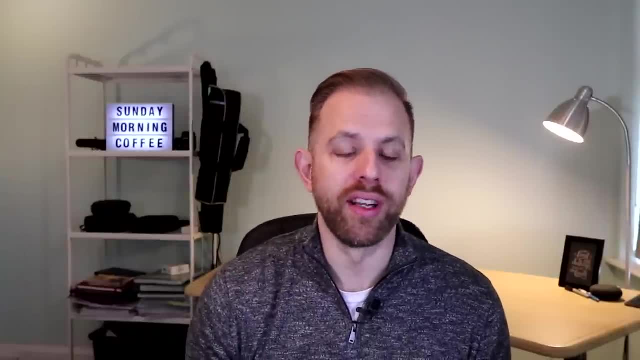 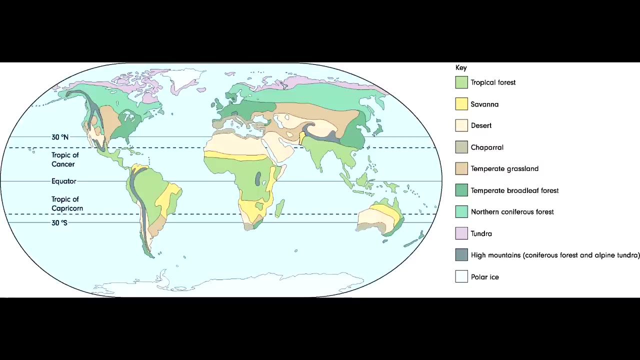 the global atmospheric circulation model to where all the ecosystems are, you should be able to spot some patterns emerging between the different latitudes, and as we move towards the north or towards the south, you can see the ecosystems changing. So, again, the global atmospheric circulation model helps us explain why we get these different ecosystems that see so. 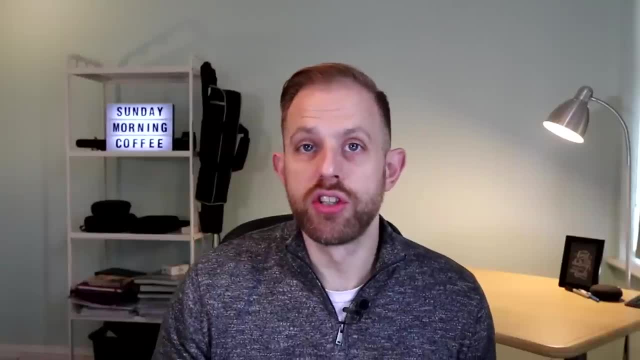 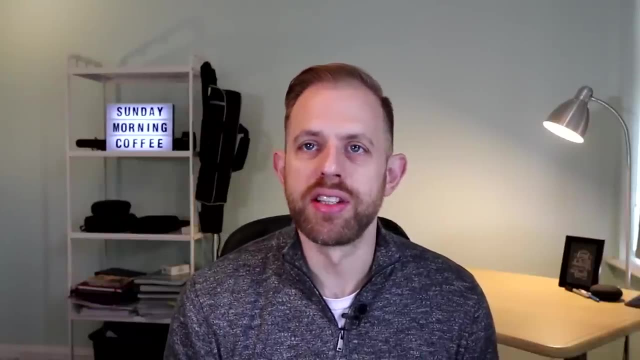 many different patterns. So this is a way of trying to explain why we get these different changes in weather and climate. So what we should see are those different boundaries, those different degrees in latitude, is we're going to see different things happening, different climates, different. 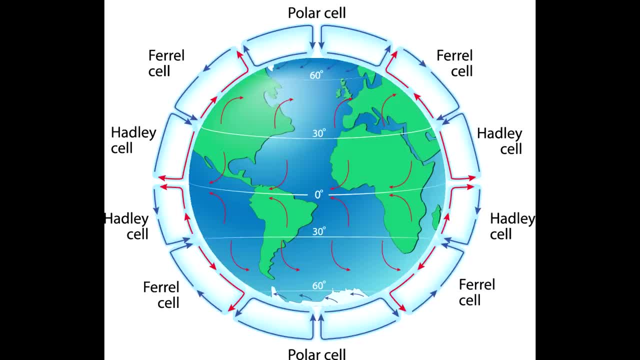 weather conditions. So we're going to break it down through that. Now we're going to look at the three main cells. It's broken down into three cells, which is called the Hadley cell, the Ferrell cell and the Polar cell, And I think at GCSE level we want to just know a little bit about those three. 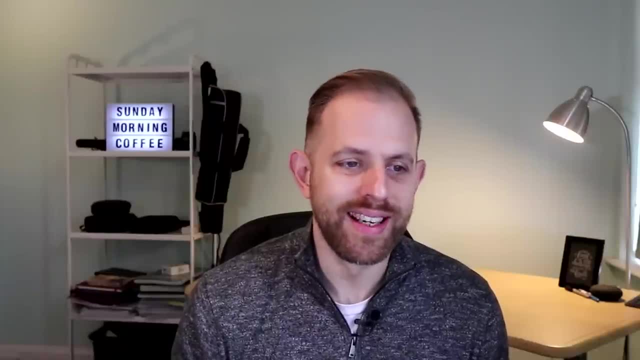 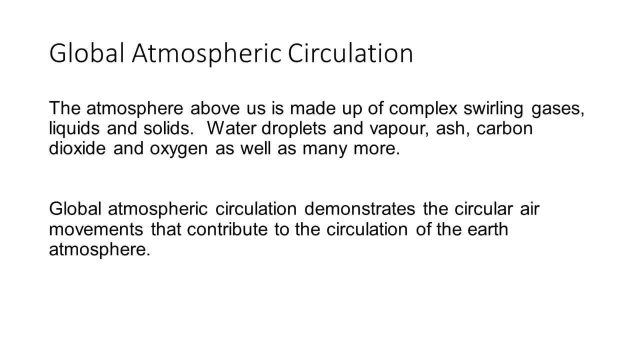 cells, what type of climate they're in and what type of climate they're in. So we're going to look at the different climates and conditions we're going to see there and try to have a simple explanation about what is actually happening in those different cells. What we see in the atmosphere is lots of 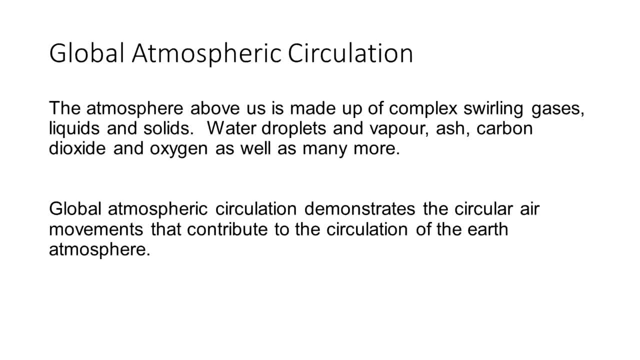 complex swirling gases and liquids and solids, water droplets and vapor and carbon dioxide and oxygen, So lots of stuff is moving around there. Global atmospheric circulation demonstrates the circular air movements that contribute to the circulation of the earth's atmosphere, So we get lots of moving parts as part of this diagram. We've got two major things happening. 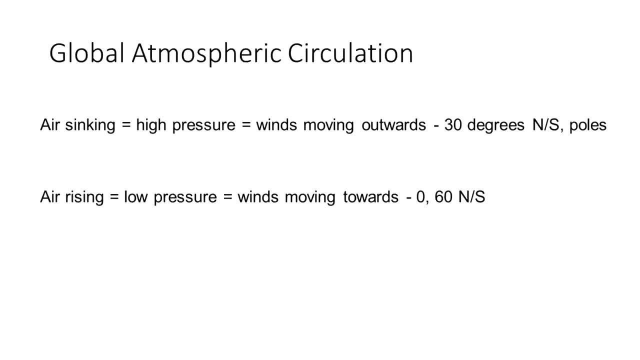 We've got air sinking and air rising. So when we see air sink, we get high pressure systems. This means we get winds moving outwards, away from those areas. But when we get air rising, we get low pressure systems. therefore, wind is moving towards. 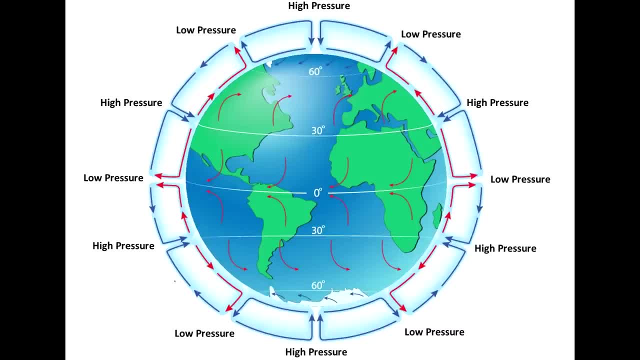 So what we see is we see air sinking at 30 degrees and the poles, which means generally a high pressure system. So when we're talking about low pressure, we've got wind moving towards that area. We've got it at zero degrees and 60 degrees Now. these are low pressure areas. so the weather. 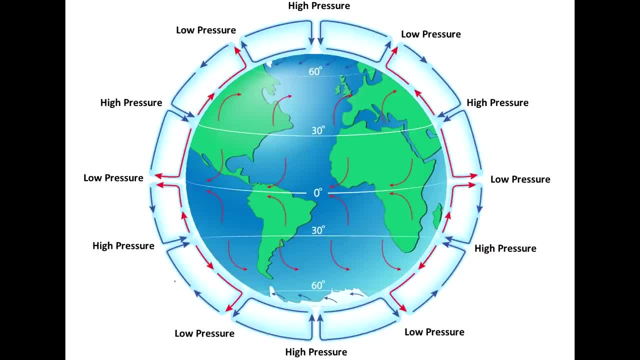 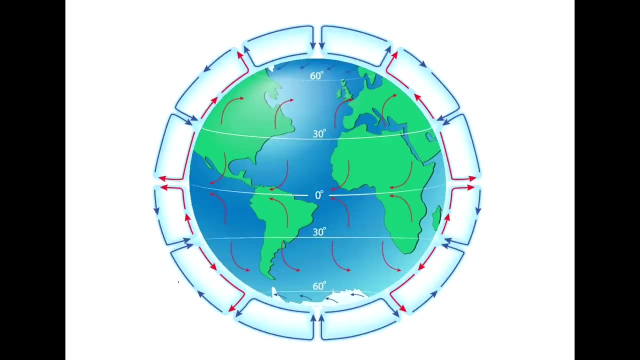 is less stable. We see lots of wind and rain and hot and humid atmospheres as well in those areas. So the winds that are labeled on this diagram in the red and the blue arrows on the actual diagram are the ones that are moving towards the low pressure areas. So we've got a lot of wind moving. 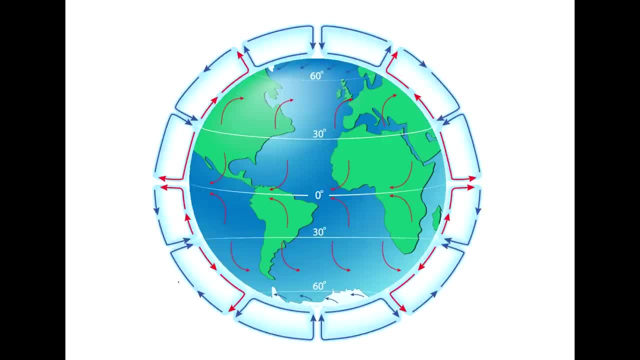 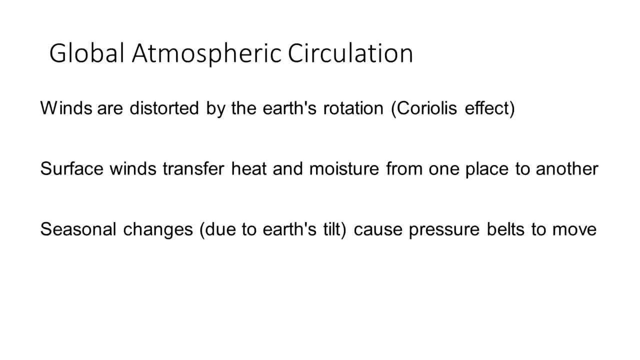 the regular sea hallow wind pattern. So wind is a diagnostic pattern distorted by the earth's rotation, also called the Coriolis effect. Surface winds transfer heat and moisture from one place to another. That's why weightолoretéo gebe tisas. 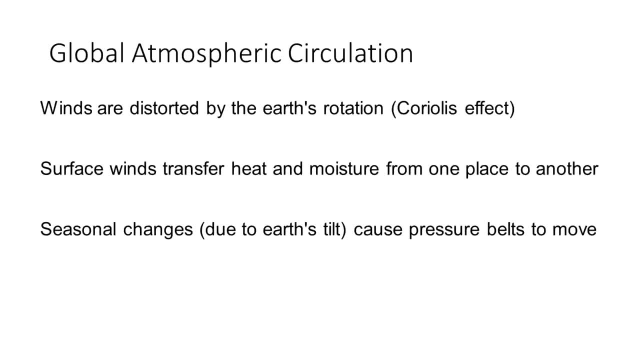 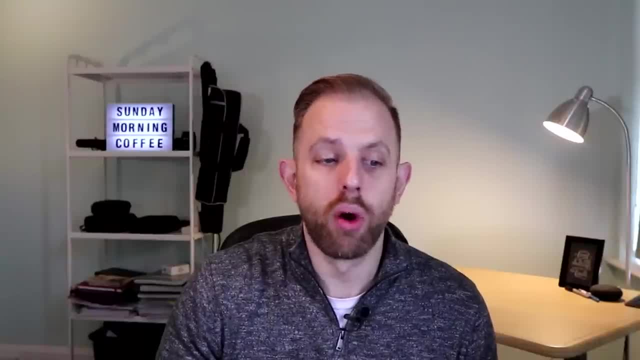 components in a global atmospheric ожидance as low as 367 общ 탈 in Vipúl. Grenade in circulation transfer heat and moisture to different places. so this is why we see differing climates around the world. so we're just going to look at the main three cells. 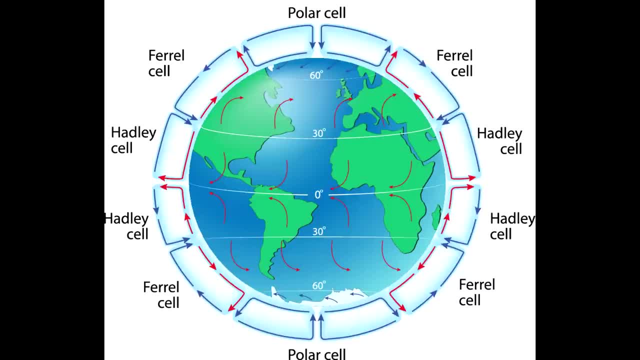 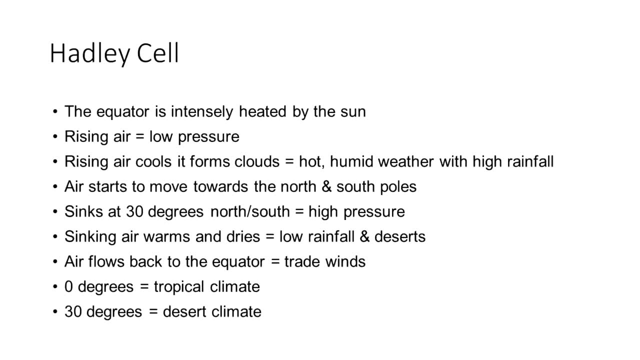 so we've got the hadley cell now. this is around either side of the equator and it gets a lot of intense heat from the sun. what we see to start with at the equator is we get lots of rising air, which is low pressure. so when we get that rising air it cools to form clouds, so we get hot, humid. 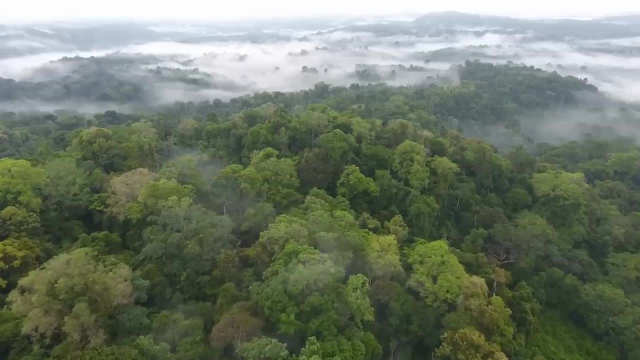 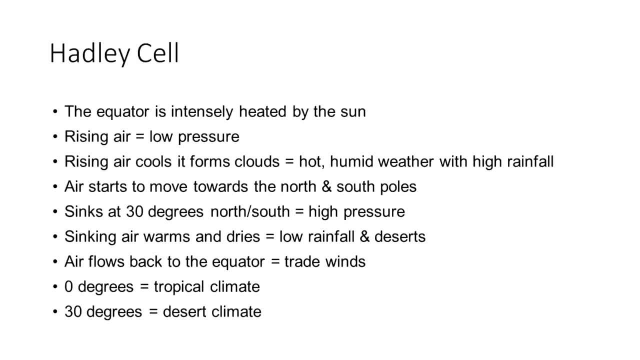 weather with high rainfall and this is where we get our tropical rainforests. then the air starts to move towards the north and south pole, so away from the equator. then it starts to sink. so we've got the sinking air, warming and drying and therefore we get our low rainfall and deserts. 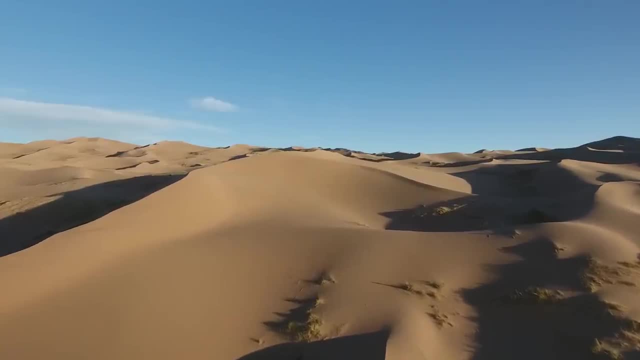 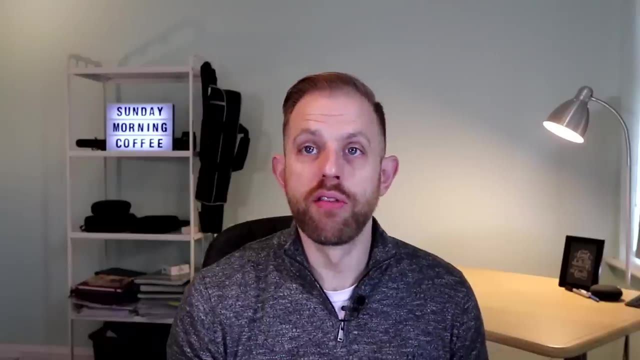 so when we get out towards 30 degrees, that is where we get our desert climates. then we get the air flowing back to the equator, which again is illustrated by the trade winds. so just to go over the hadley cell, we see generally at zero degrees or just either side of the equator we've seen. 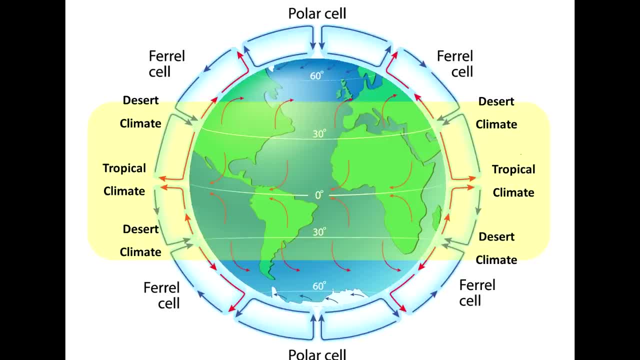 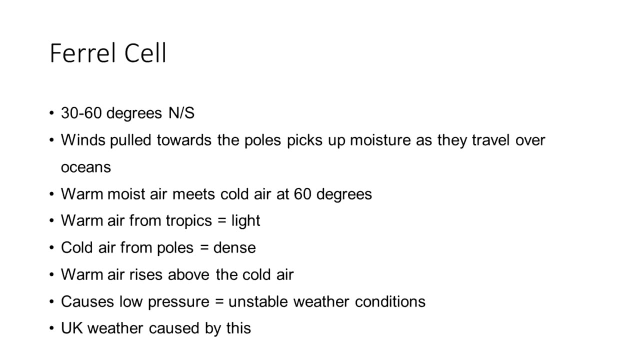 tropical climates: hot and humid, with lots of rainfall. and as we move away from the equator towards 30 degrees, that's where we see desert climates. the ferrule cell again. this is between 30 and 60 degrees north and south and what we see is the wind pulling towards the poles and that. 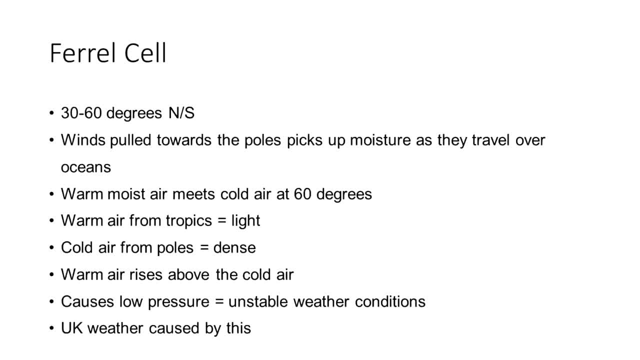 picks up the moisture as it travels over some of the oceans. when the warm, moist air meets cold air, that's when we start to get those mixing of warm and cold air. so we get this mixture of warm air from the tropics, which is quite light, and cold air from the poles, which is quite dense. now what we see? 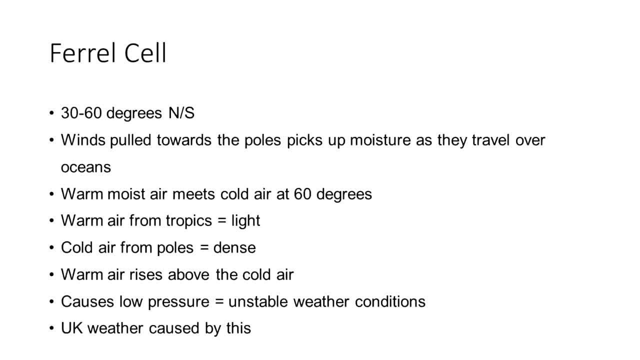 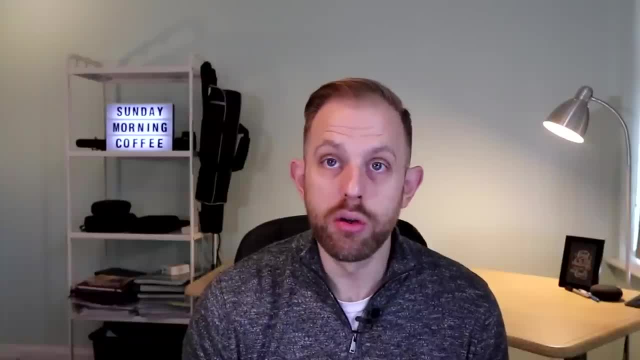 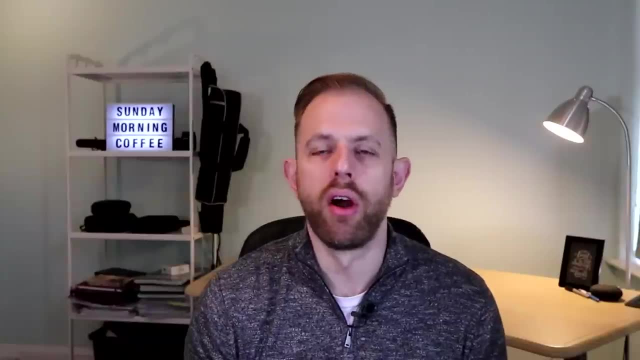 is that light warm air rises above the cold air and this causes a low pressure system, so we get really unstable weather conditions. now the uk is within this cell, so this really explains why we see such differing weather and we get lots of low and high pressure systems around the world. 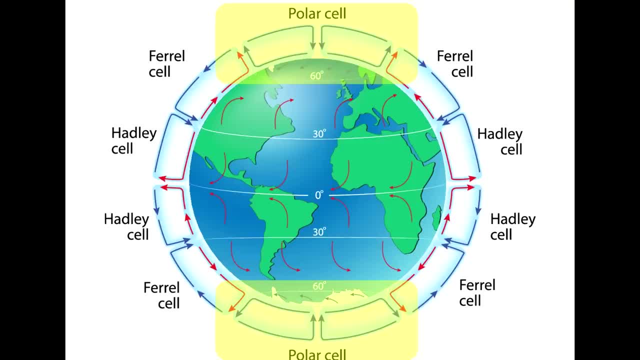 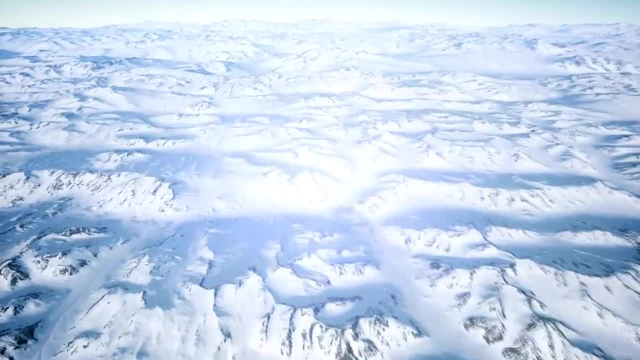 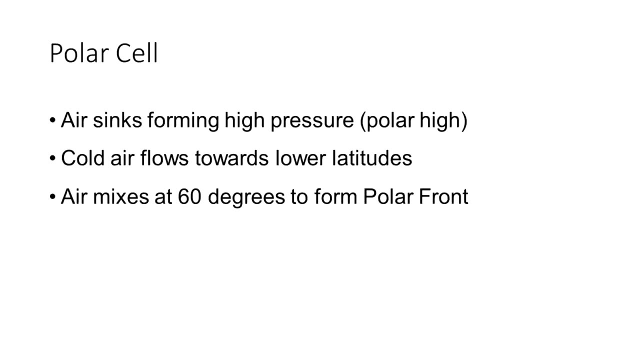 throughout the year. and lastly, we've got the polar cell. so we've got that air sinking to form a high pressure system which is called a polar high. at the poles, cold air flows towards the lower latitude, so it moves away from 90 degrees north and south and then it starts to mix with 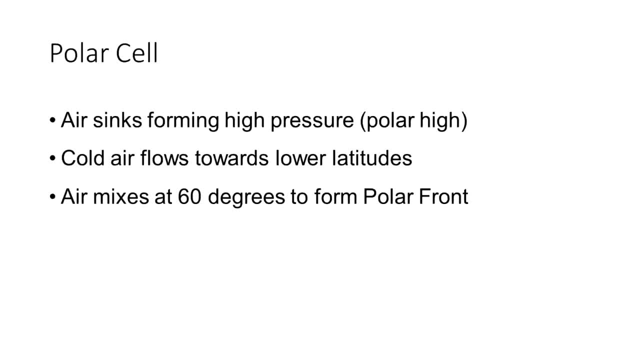 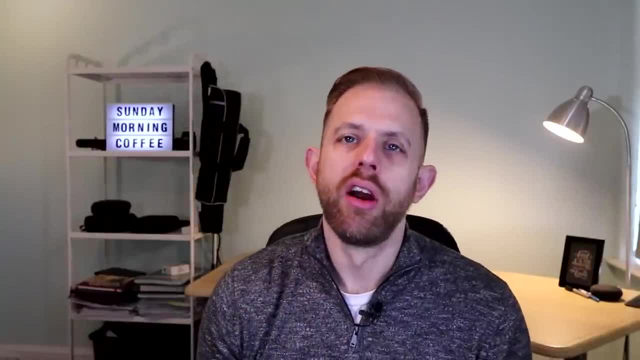 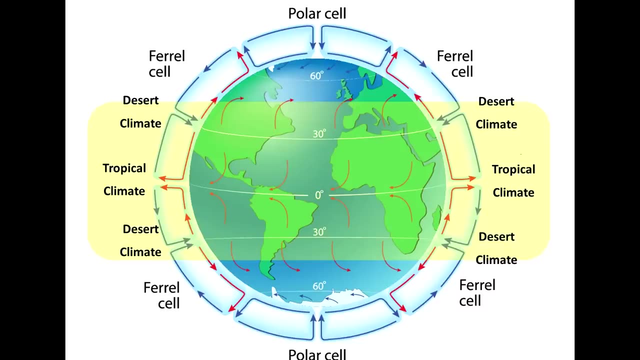 those, those other air types, at 60 degrees to form a polar front. so the main things to take away from this model, if we're going to try and break it down into really small parts: understand the different types of climates we see at each cell. so again, the hadley cell, between zero and 30 degrees. 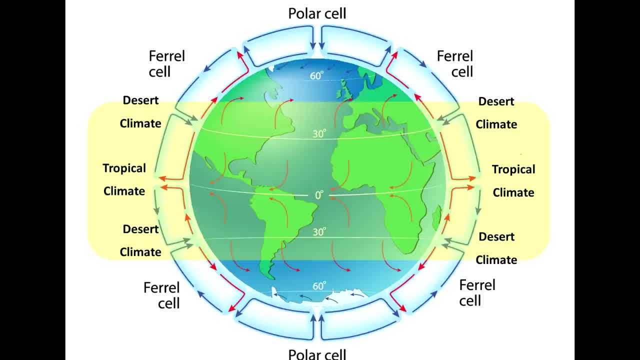 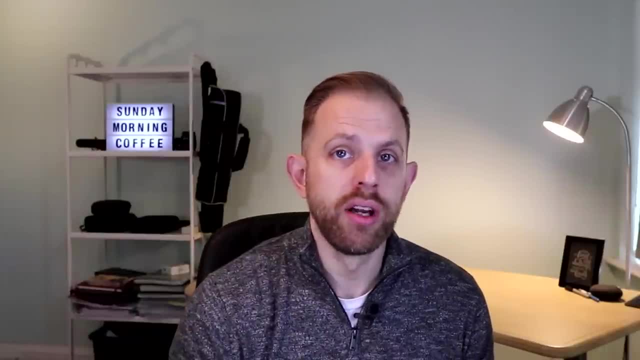 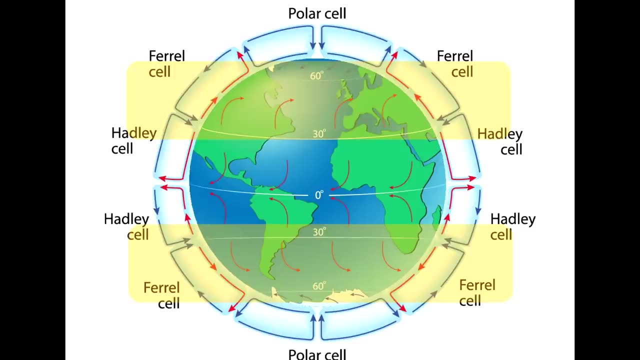 we see tropical climates around the equator and as we move away it transfers into desert environments which are very dry and hot. when we move on to the feral cell we see very changeable conditions, lots of air mixing and that's why in the uk we get lots of changeable weather. 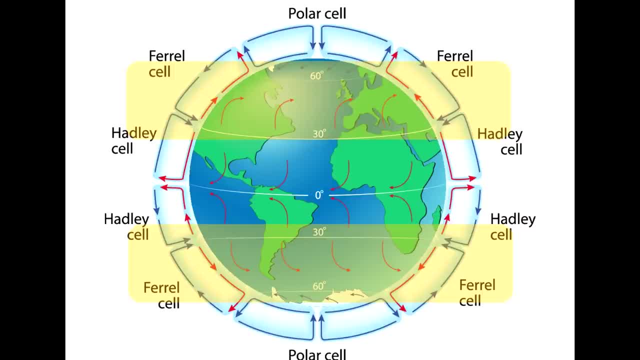 lots of rain, lots of hot times as well, and then it's just very unstable and it's very difficult to forecast what type of weather we're going to get in the future. and then, lastly, we've got the polar cell between 60 and 90 degrees. we get that cold air moving away. 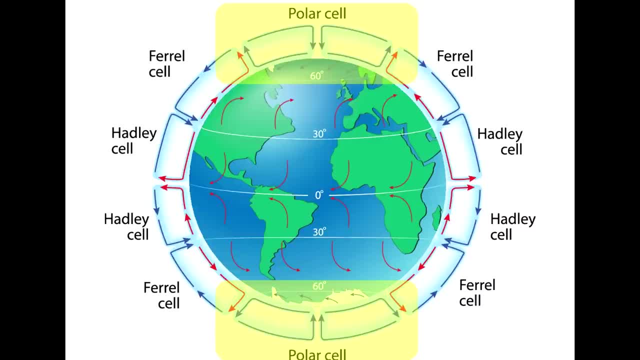 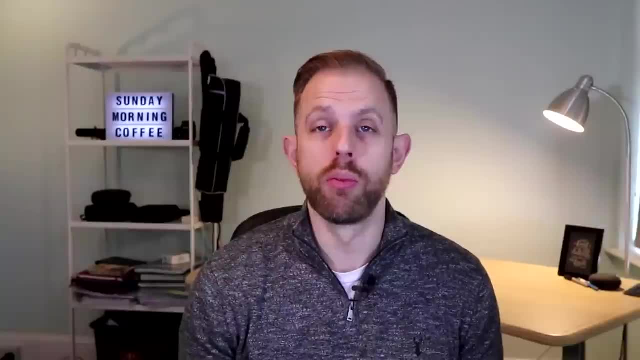 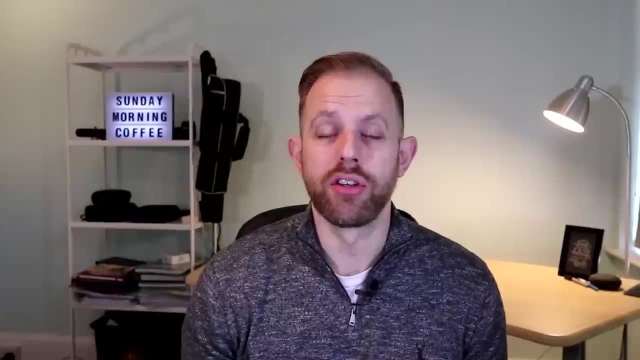 from the poles, transferring that cold air down towards the lower latitudes. so that is a quick summary of global atmospheric circulation. i hope it's been a really useful breakdown and i've done a good job of breaking it down into those smaller chunks, if you find. if you want to find out more about the subject, then go check out some of the links i'm 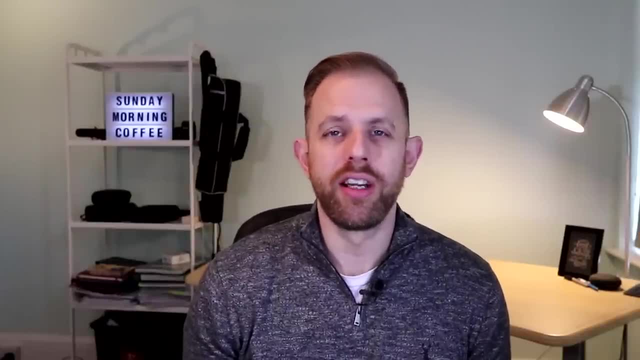 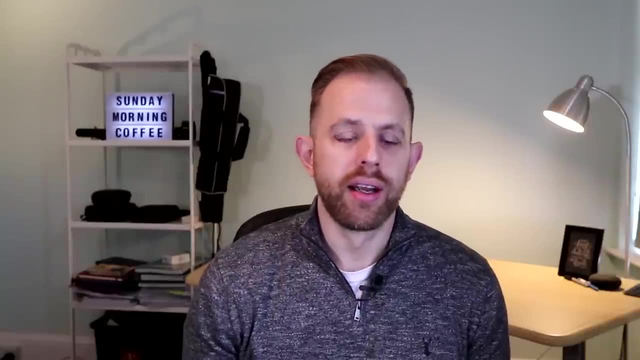 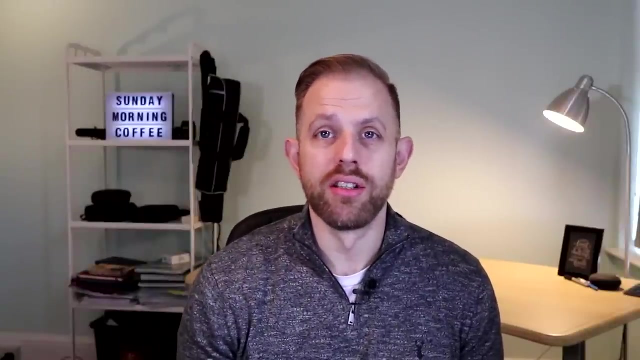 going to include in the description. and lastly, if you found the video useful, please give it a like and subscribe to the channel, just to let me know whether this has actually been valuable or not. okay, next week i'll be starting to look at tropical storms, so make sure you subscribe to get that straight into your feed.